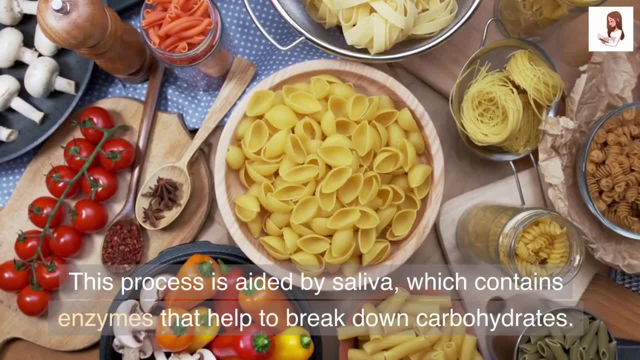 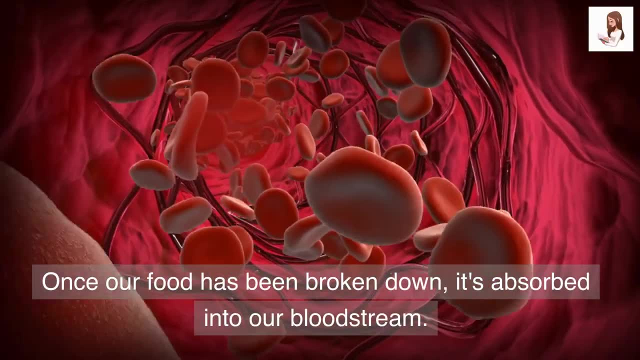 that our bodies can absorb the nutrients. This process is aided by saliva, which contains enzymes that help to break down carbohydrates. Once our food has been broken down, it's absorbed into our bloodstream. The nutrients are then transported to our cells, where they're used. 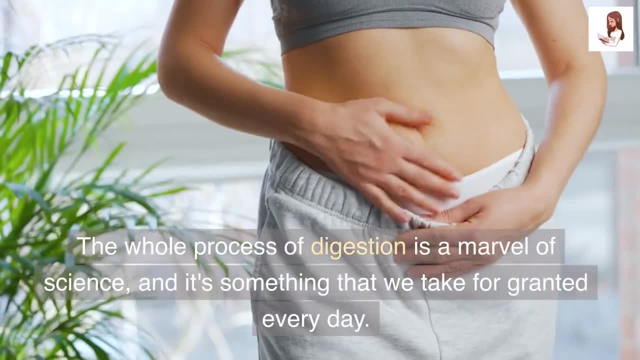 for energy. We're not just taking in nutrients, We're also interacting with a complex system of chemistry and physics. For example, when we chew our food, we're breaking it down into smaller particles or stored for later use. The whole process of digestion is a marvel of science, and it's 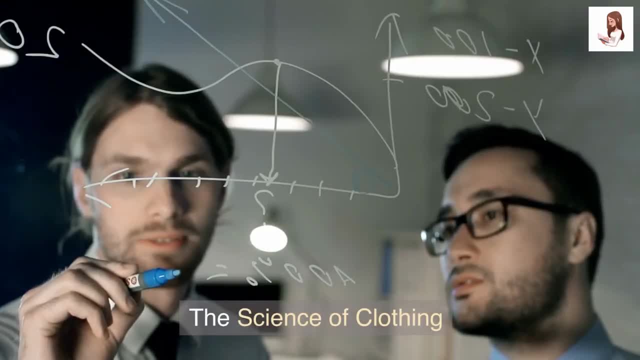 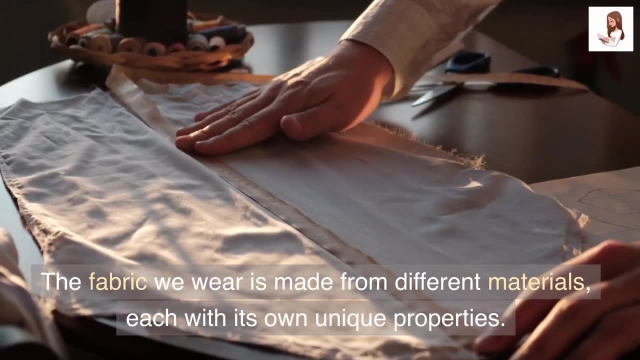 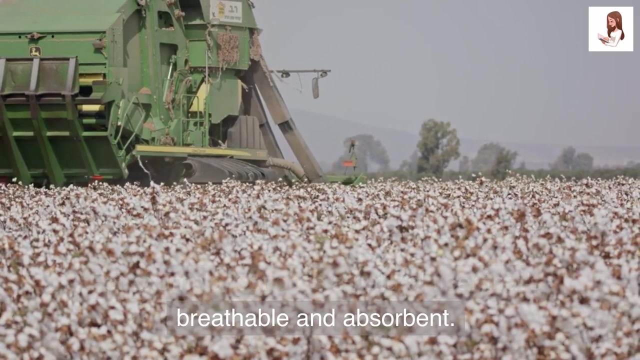 something that we take for granted every day: The science of clothing. Another everyday thing that's full of science is clothing. The fabric we wear is made from different materials, each with its own unique properties. For example, cotton is a natural fiber that's breathable and 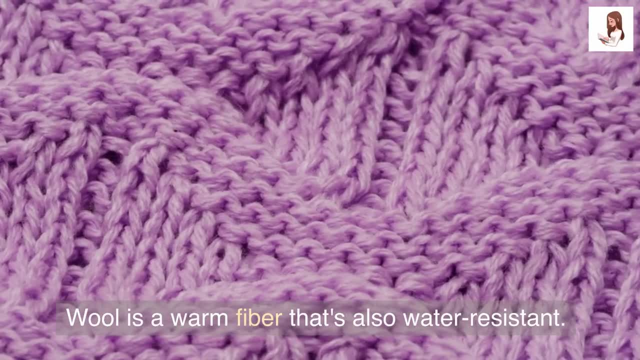 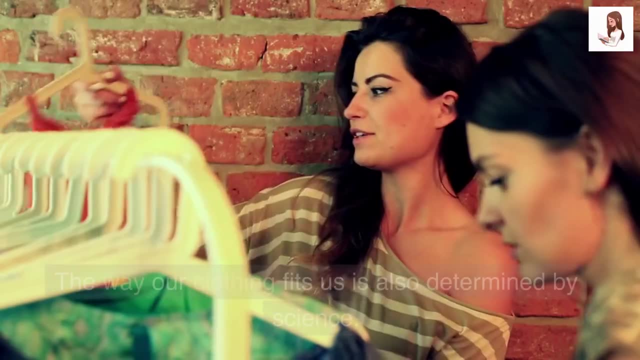 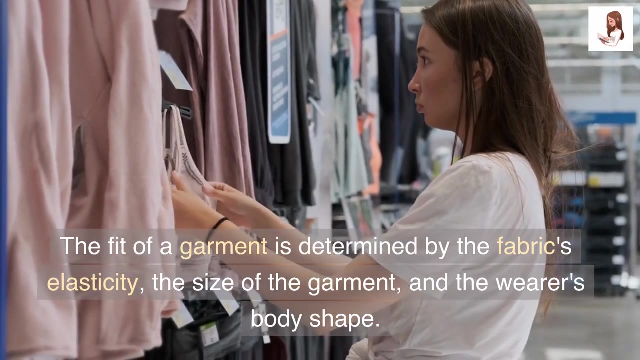 absorbent. Wool is a warm fiber that's also water-resistant, And polyester is a synthetic fiber that's wrinkle-resistant and easy to care for. The way our clothing fits us is also determined by science. The fit of a garment is determined by the fabric's elasticity. 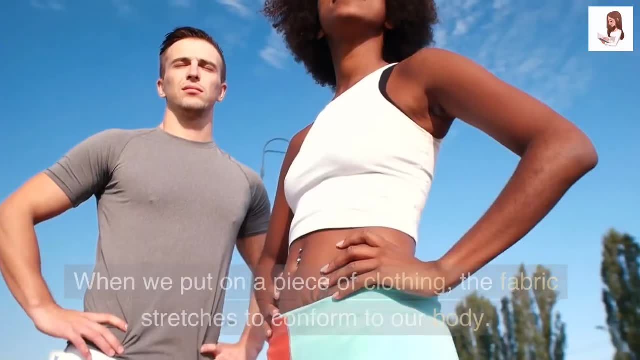 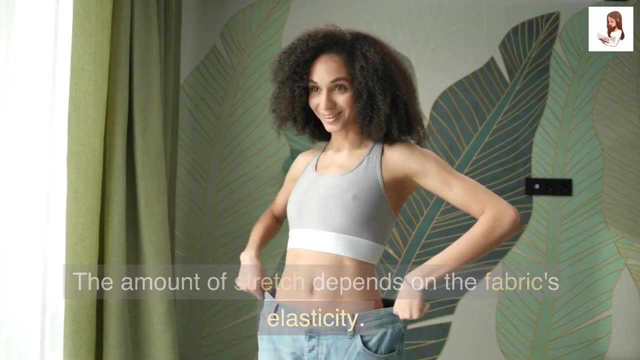 the size of the garment and the wearer's body shape. When we put on a piece of clothing, the fabric stretches to conform to our body. The amount of stretch depends on the fabric's elasticity. The science of transportation: Finally, let's talk about transportation. 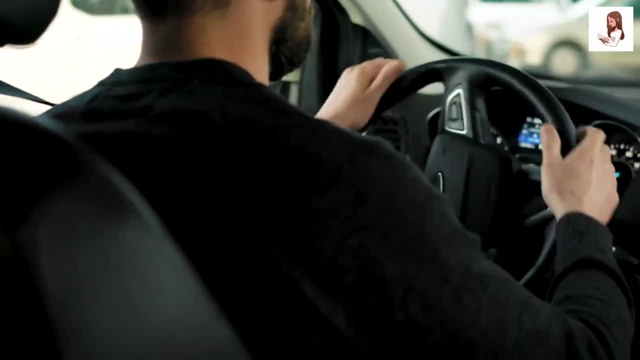 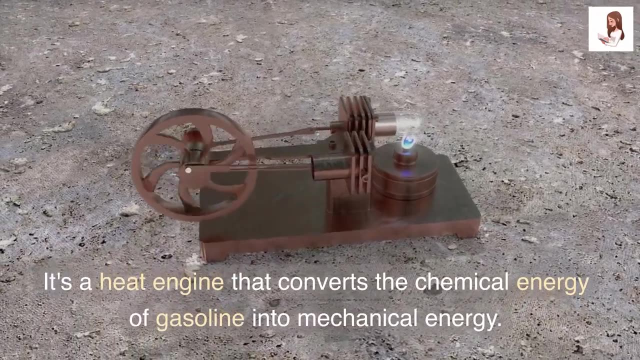 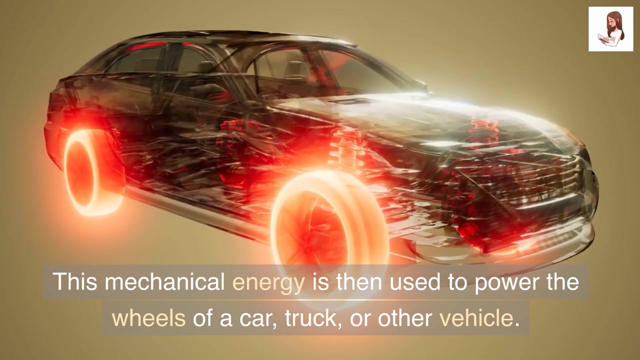 The way we get around is also a product of science. For example, the internal combustion engine is a marvel of engineering. It's a heat engine that converts the chemical energy of gasoline into mechanical energy. This mechanical energy is then used to power the wheels of a car. 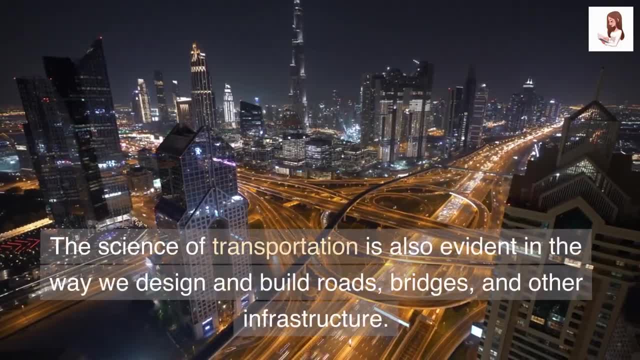 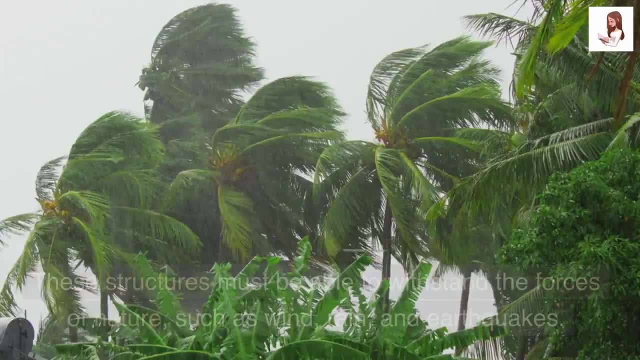 truck or other vehicle. The science of transportation is also evident in the way we get around. The way we get around is also a product of science, For example, the way we design and build roads, bridges and other infrastructure. These structures must be. 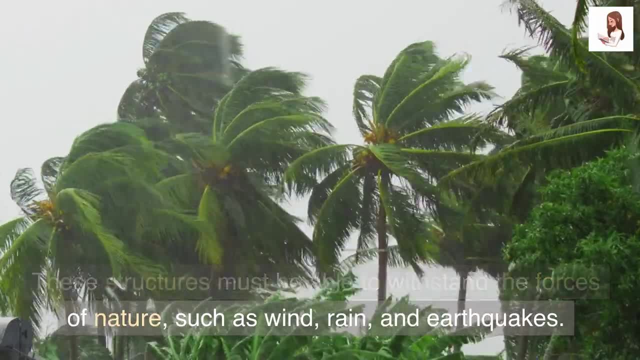 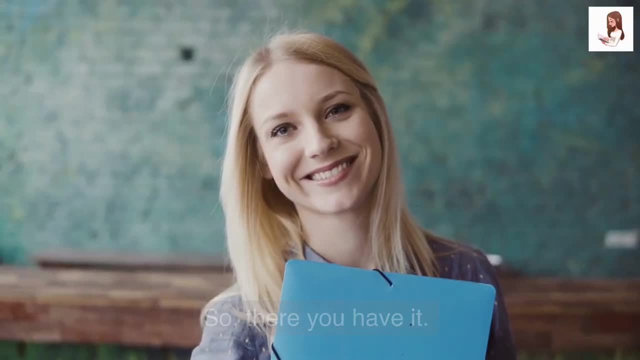 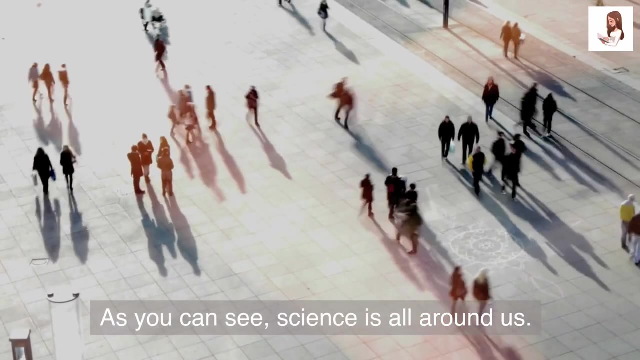 able to withstand the forces of nature such as wind, rain and earthquakes. They must also be safe for people to use. So there you have it, A brief overview of some of the science behind the things we use every day. As you can see, science is all around us. It's in the food we eat.